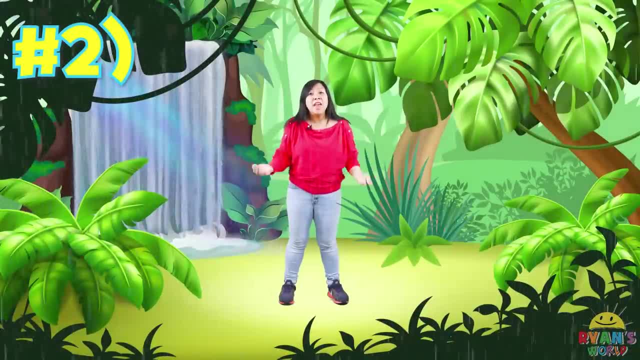 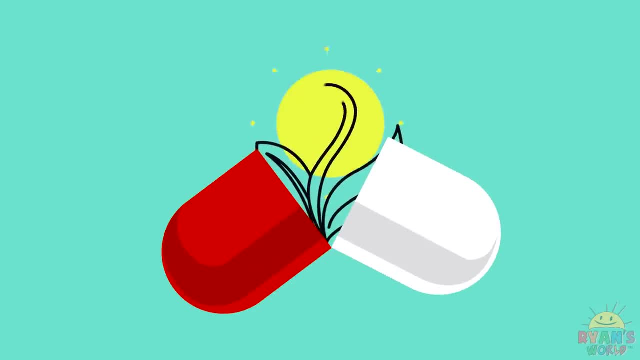 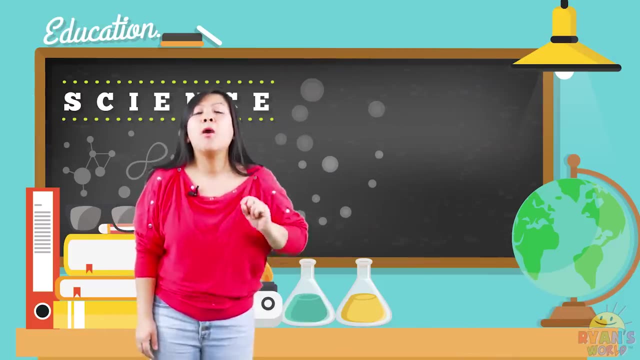 There are a couple things that I killed off in this video. plants Number two, then the plants wouldn't exist, Bye, bye. plants Number three, then we wouldn't have plants to make our medicine. Oh no, what could we do to help? I know one thing that we can do. 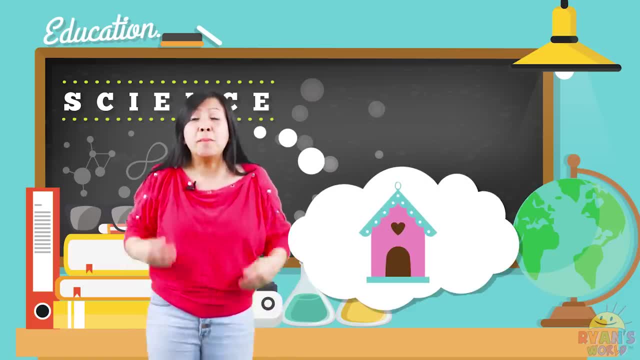 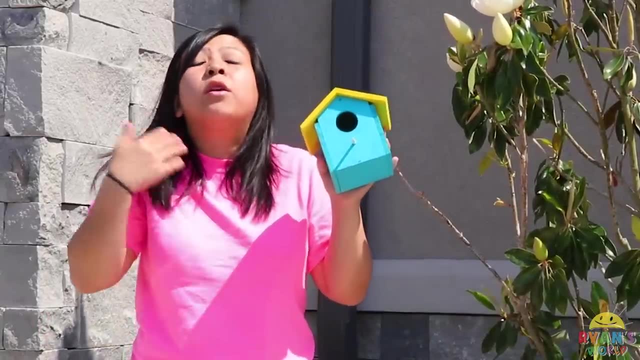 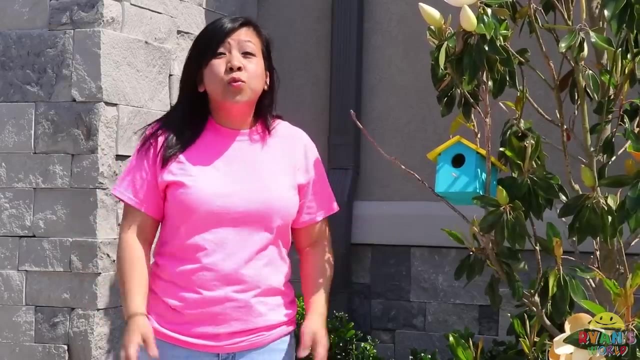 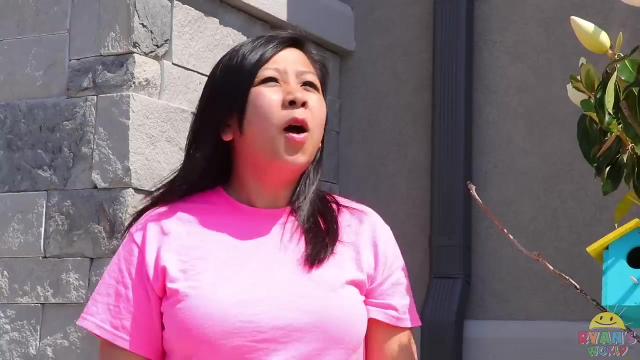 is build a home for animals that are migrating, Come on. So if you put a birdhouse like this one here, it will be a great help for birds who are migrating. We can help them get to where they need to go next, and it will make their job easier. traveling and pollinating the plants, Oh look. 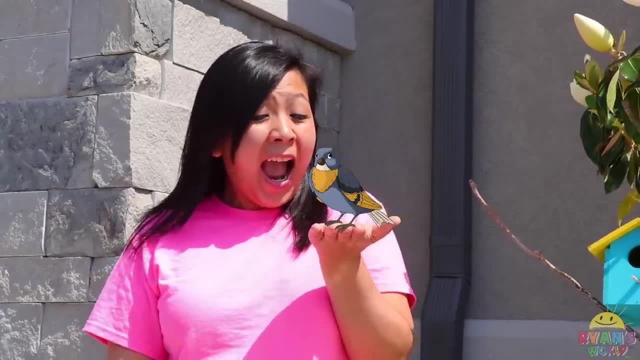 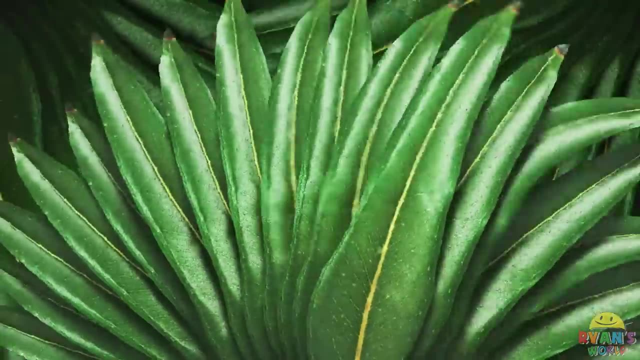 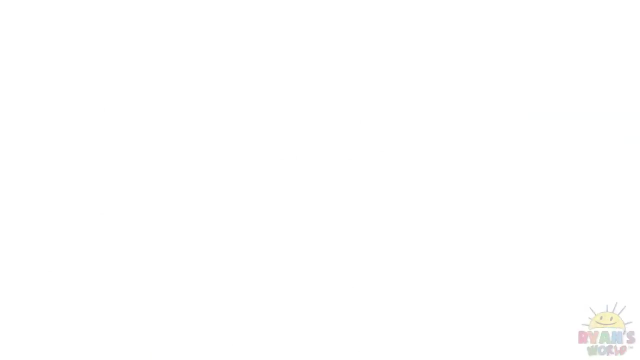 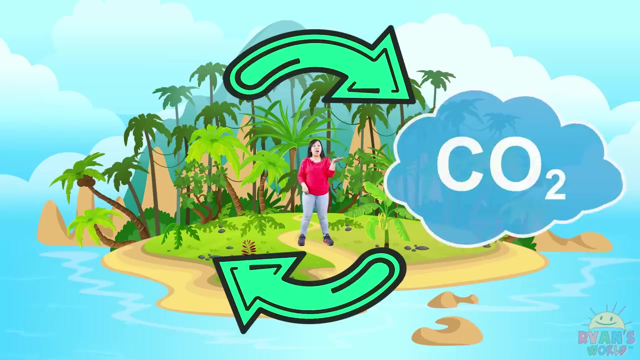 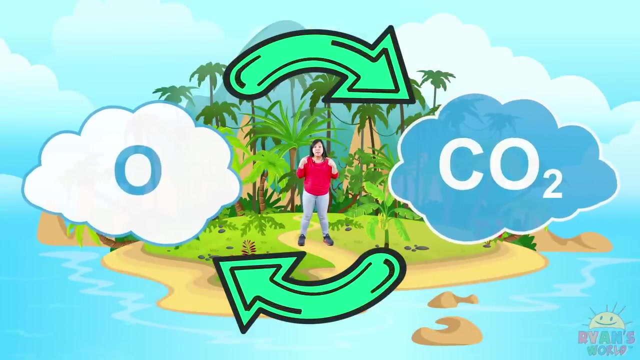 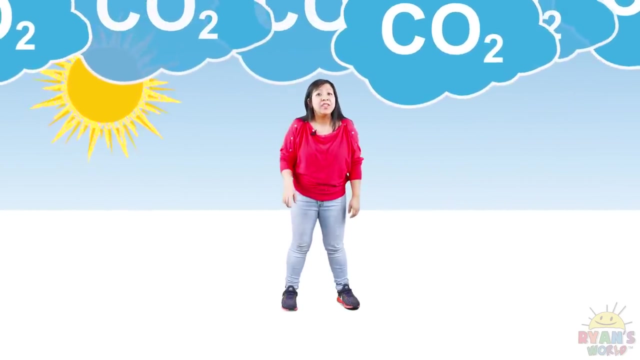 Hi. We also need the rainforest to help. It will help us stop the ice cap from melting. Rainforests are full of trees that clean our air by converting carbon dioxide, which is what we breathe out, into oxygen, which is what we need to breathe, And if we have too much carbon dioxide in the air, the temperature. 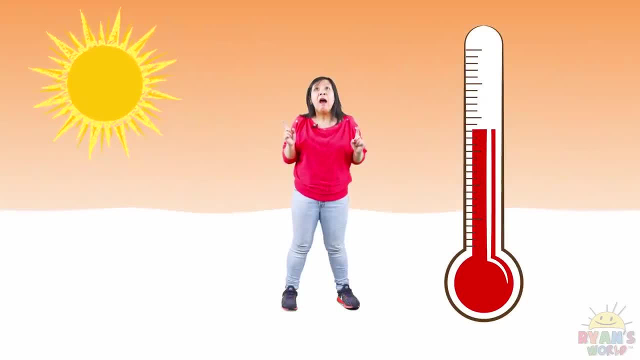 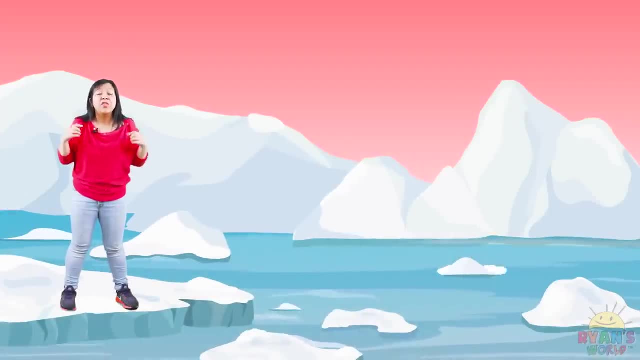 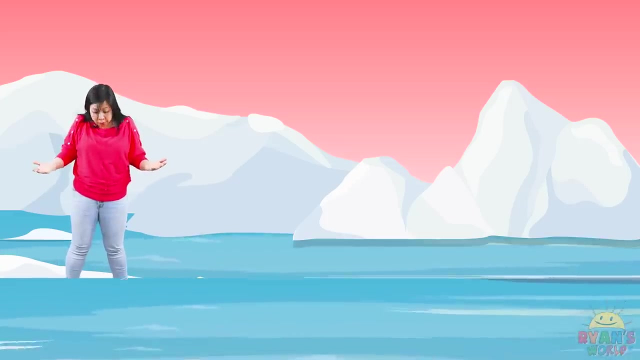 of the planet will rise. Look, Oh, it's getting hot. And if the temperature of the planet rise, the ice cap will melt into the ocean And then the ocean level will rise. Oh no, the water is rising. Oh, let's get out. 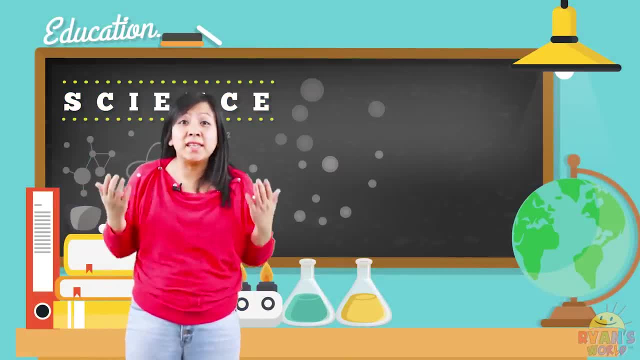 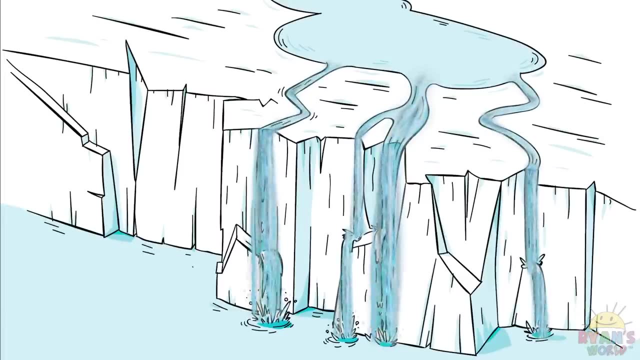 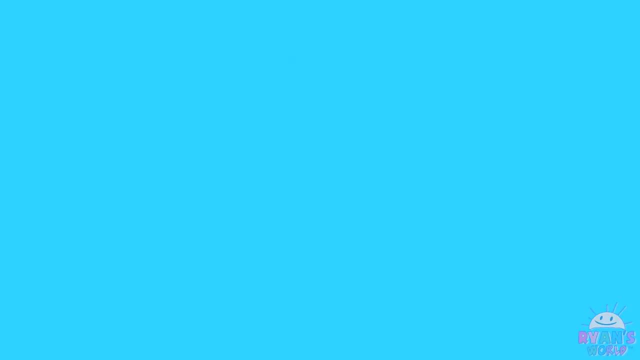 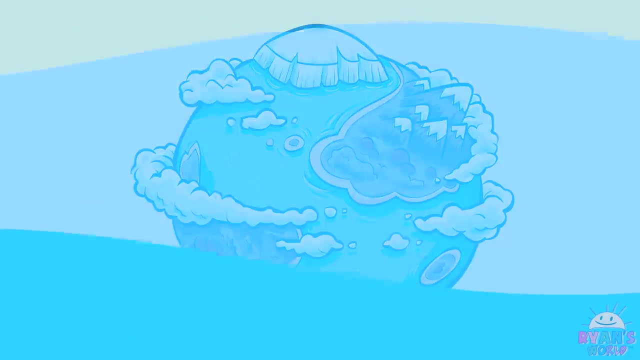 So what will happen if we let the ice cap melt? Number one: water from the ice cap will drain into the ocean. Number two: the ocean level will rise. And number three: land around the coast and land at sea level will be covered. 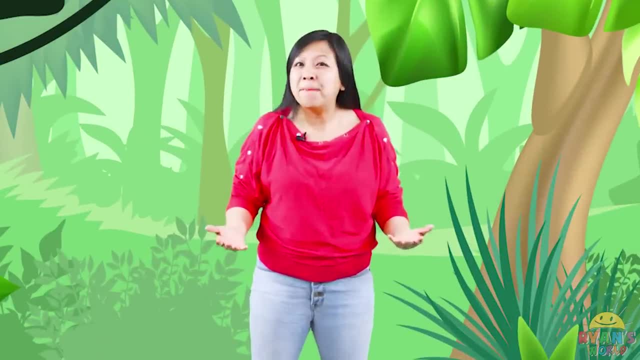 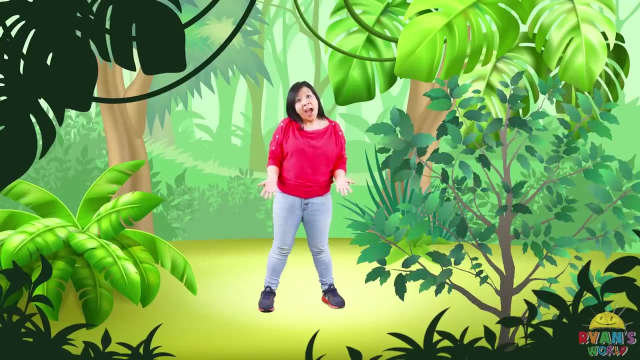 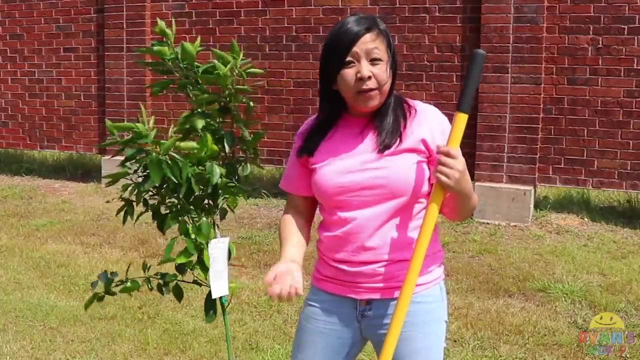 Wow, That will be a lot of water, but don't worry. One of the things we can do is plant our own tree. Let's go So. planting trees by rain water, by plenty like this one, helps both the ice cap and the rainforest. this tree over here will help convert. 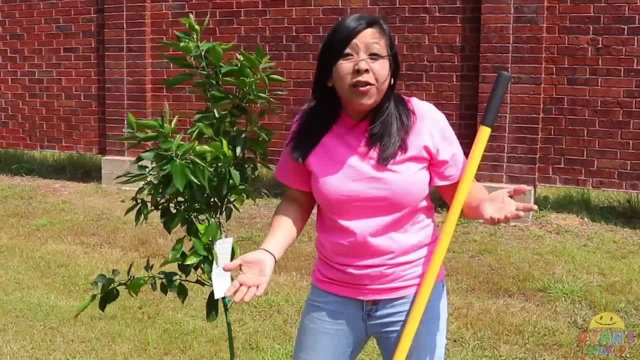 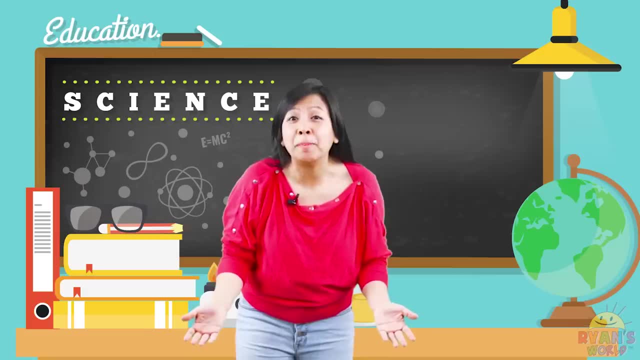 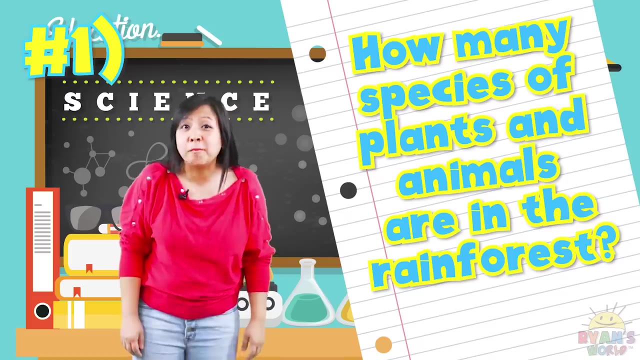 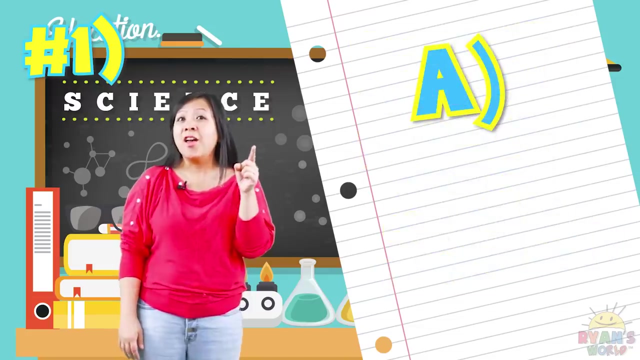 carbon dioxide to oxygen, just like all the trees in the rainforest. it's something that everyone can do, even you. thanks for helping me plant a tree. now it's time for a pop quiz, number one: how many species of plants and animals are there in the rainforest? is it a 30 million? is it b? 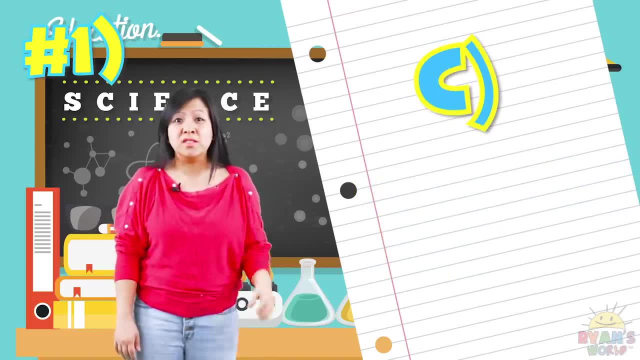 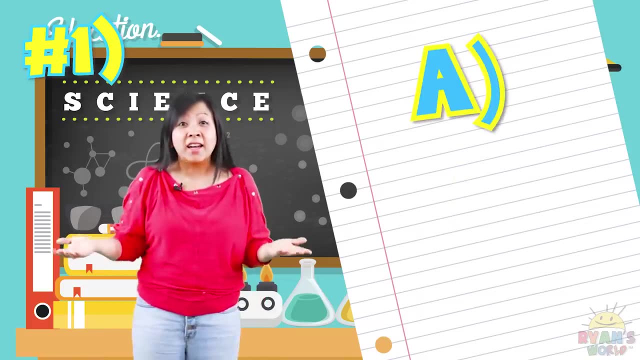 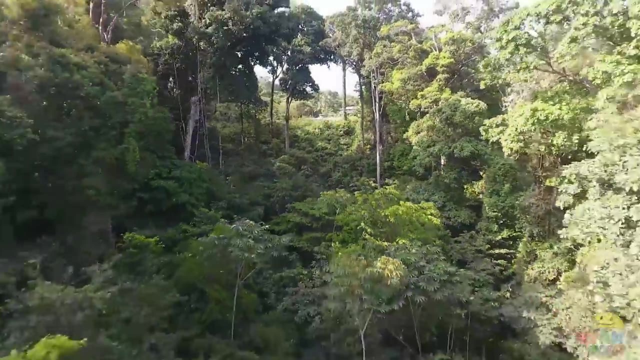 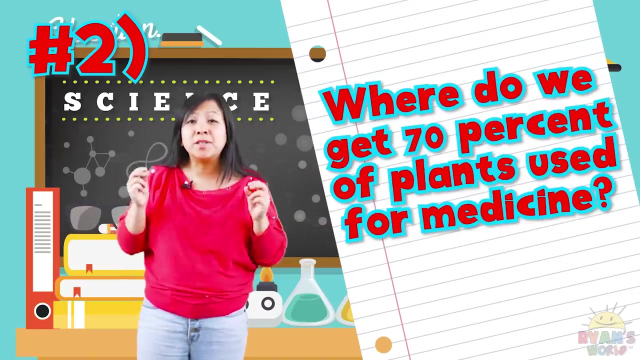 five, or is it c? zero plants and animals in the rainforest. did you guess it? it is a 30 million different plants and animals that are in the rainforest. that's a lot. question number two: where do we get 70 percent of plants we use for medicine? 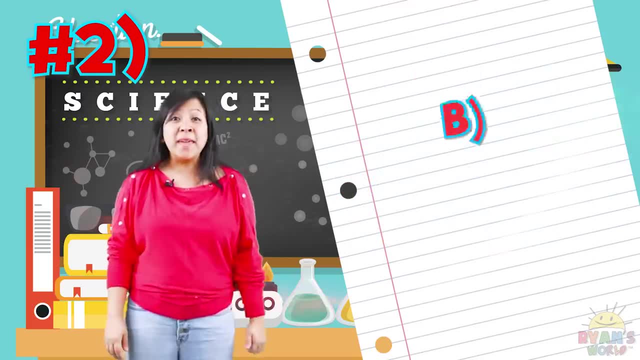 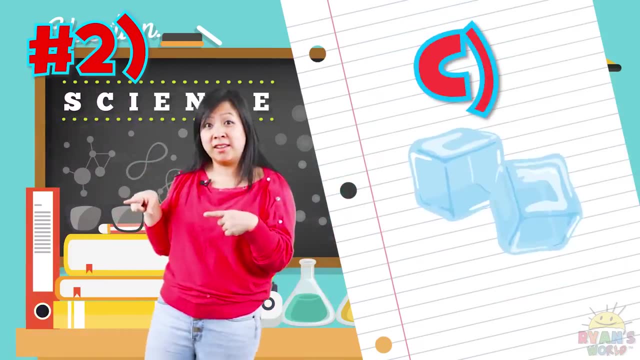 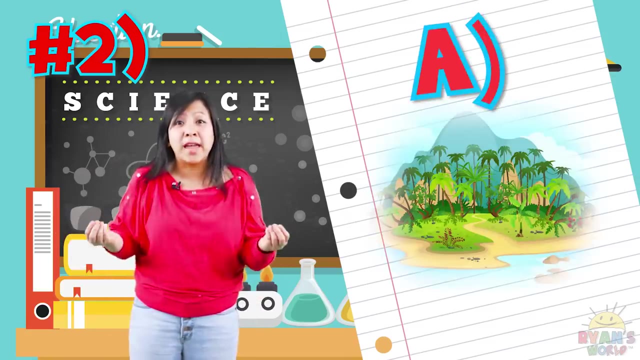 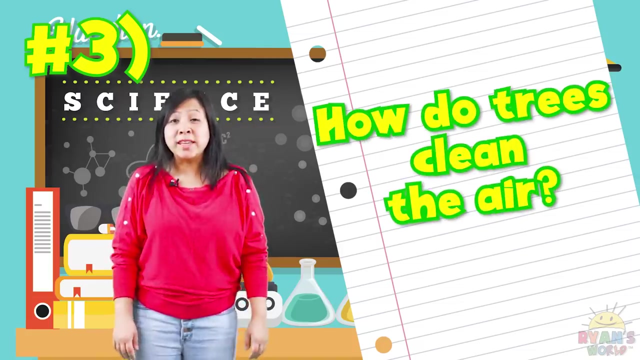 is it a the rainforest, is it b the rainbow, or is it c- ice? did you guess it? it is a the rainforest. that is where we get 70 percent of our plants that we use for medicine. question number three: how do trees clean the air that's around us? 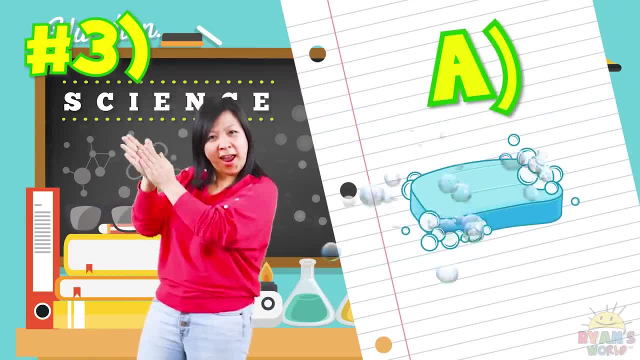 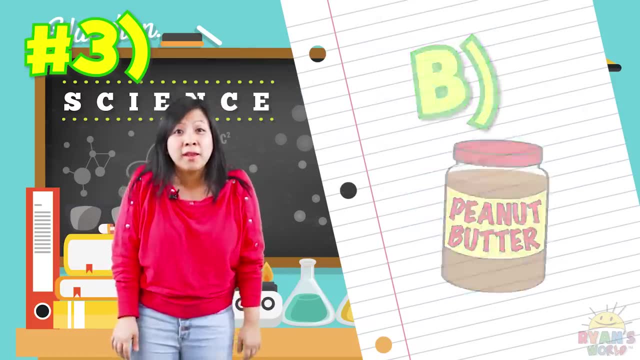 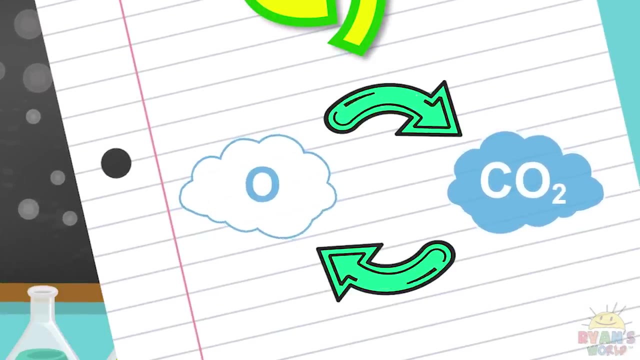 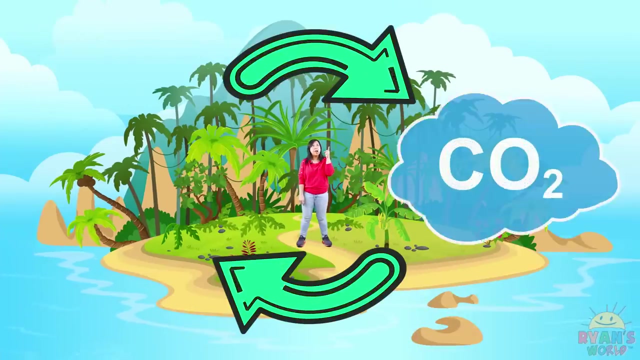 is it a with hand soap? is it b with peanut butter? oh, i love peanut butter, they're so yummy. or is it c- by converting carbon dioxide into oxygen? did you get the right answer? c- by converting carbon dioxide into oxygen. b- by converting the air that we breathe into oxygen. c- by converting the air that we breathe into oxygen. 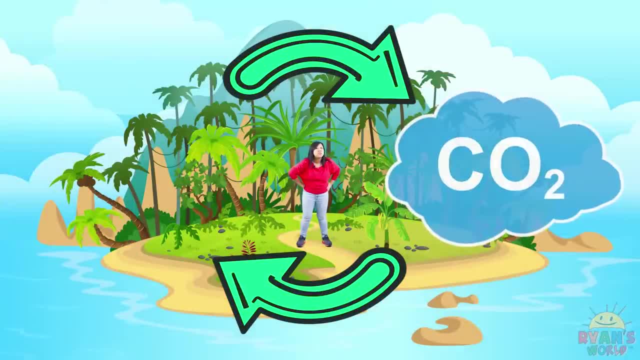 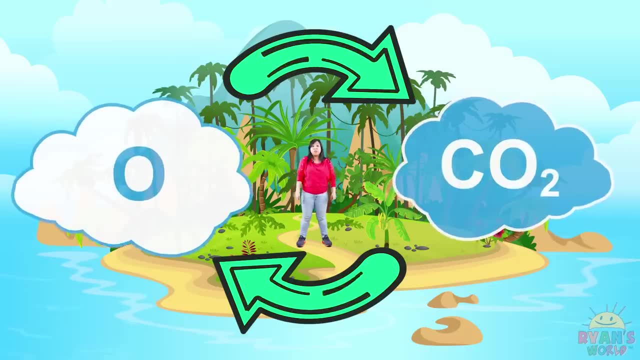 which is what we breathe out, which is the stuff that's not really good for our body. c- by converting the air into oxygen, into oxygen, which is what we need to breathe in to our body to survive. congratulations, good job, and if you didn't guess it all right, you can try again next time. so now that we learned so much about ways to save the planet, we can start off by sharing it with our friends and friends. so go ahead and give it a big thumbs up if you liked it. do check out our channel for more great videos like this one and do subscribe, if you haven't already, and leave us a comment below and let us know if you have any questions back there. 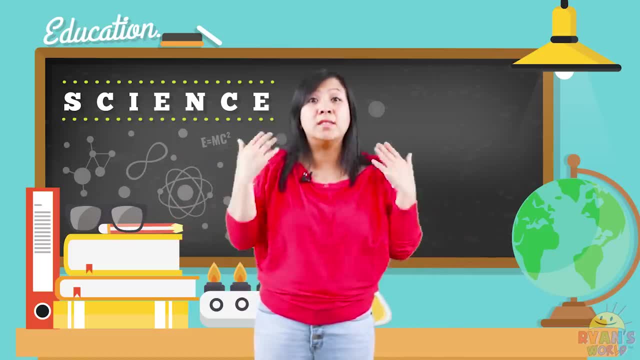 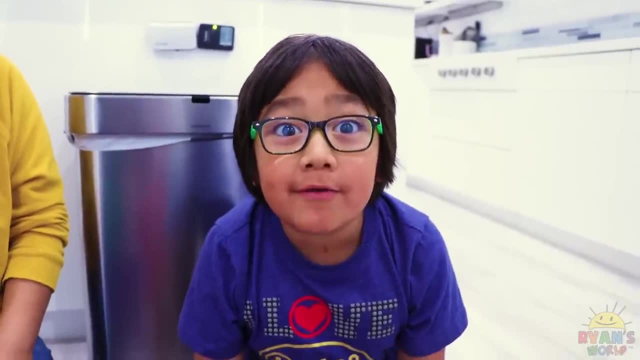 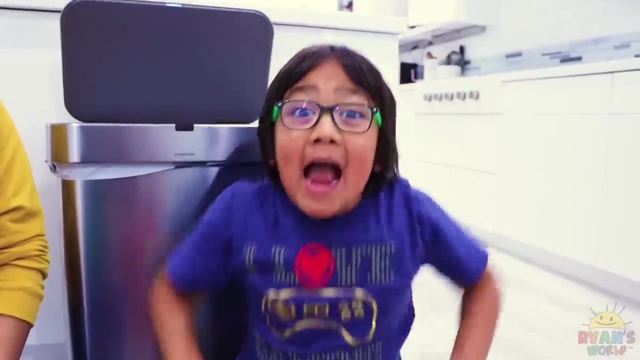 now that we learned so much about ways to save the planet and be a part of our life about ways to save the planet, let's go back and tell Ryan: I hope you guys learned a lot of ways to save the planet. bye, remember, or stay happy and rise up. bye, I'm gonna go save the planet more. you.